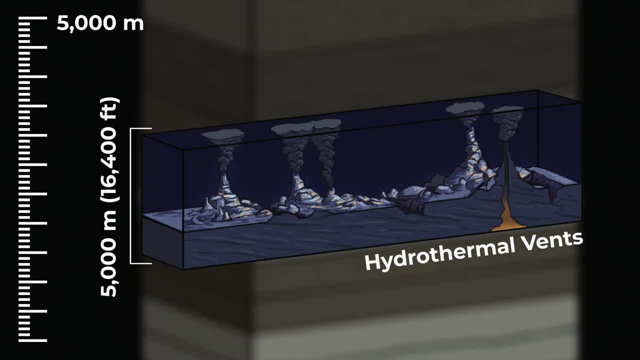 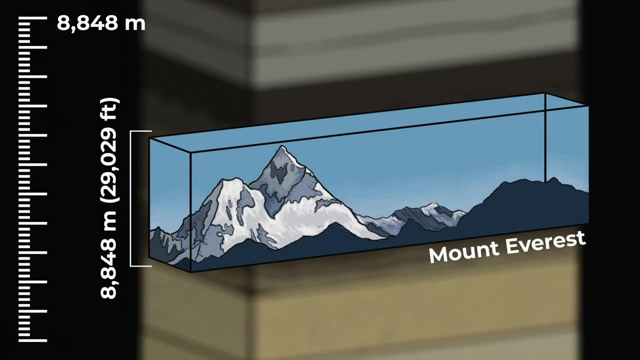 These vents are formed by deep cracks in the ocean floor, where seawater gets caught, becomes superheated and is forced back up. The tallest above-sea-level mountain in the world is Mount Everest and if it were underground, its tip to base would reach a depth of 8,848 meters or 29,029 feet. 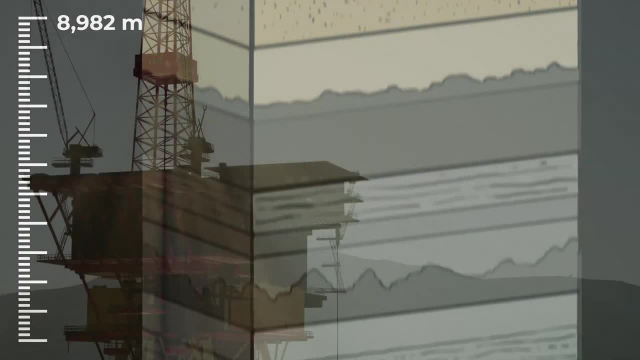 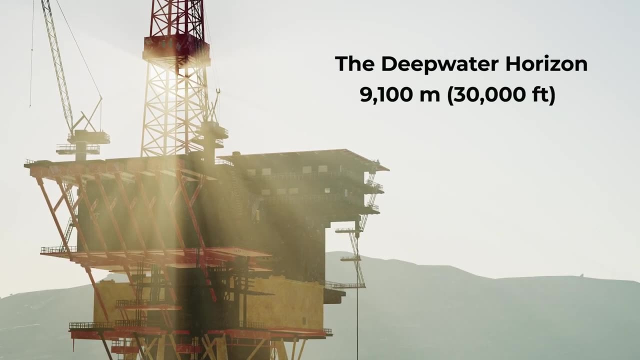 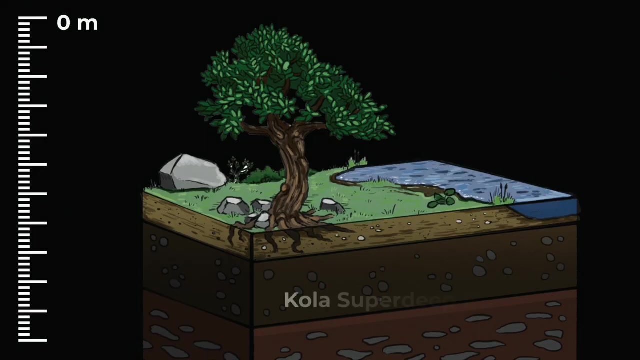 The Deepwater Horizon was an oil drilling rig that was placed out in the ocean to drill for oil. It drilled as deep as 9,100 meters, or 30,000 feet, before it exploded in 2010.. The Kohler Superdeepwater. 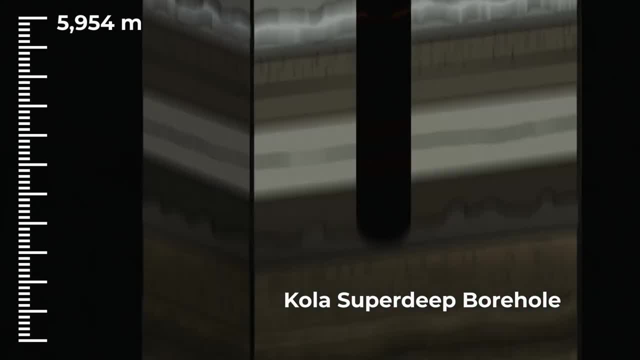 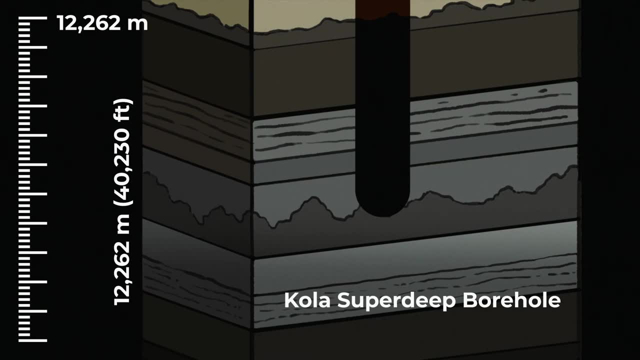 created as a scientific drilling project by Soviet geologists, reached a depth of 12,262 meters, or 40,230 feet, before the project had to be abandoned in 1992.. That's when the temperature at that depth got too hot for the drill. 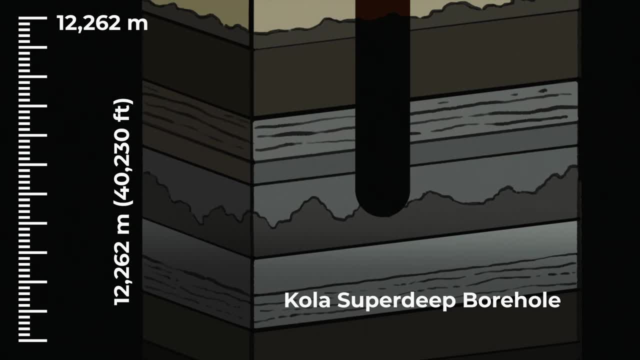 The borehole took almost 20 years to dig and it earned the title of the deepest human-made hole. However, in 2012,, the borehole became the deepest human-made hole in the world. In 2012,, the Z-44 Shavio well was completed by the oil and gas company Exxon. 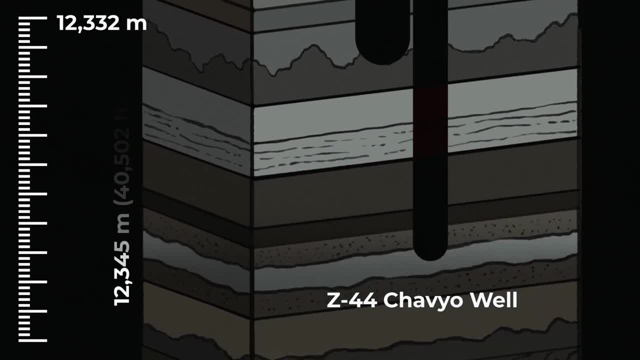 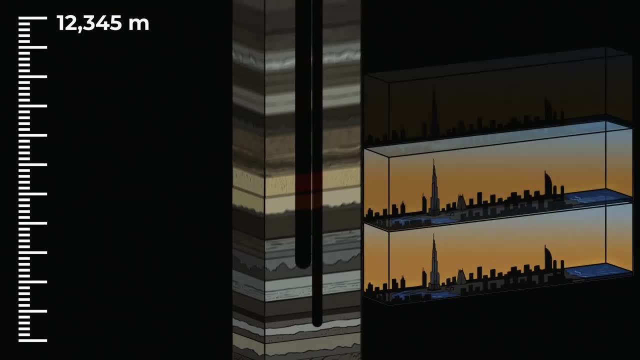 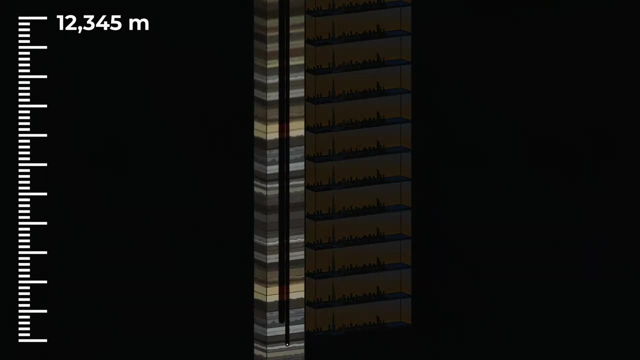 and it became the deepest well on Earth. It is 12,345 meters, or 40,502 feet, and it would fit about 15 of the Burj Khalifa buildings stacked on top of each other. Even at this deepest point of this human-made hole, we're still not even close to the mantle. 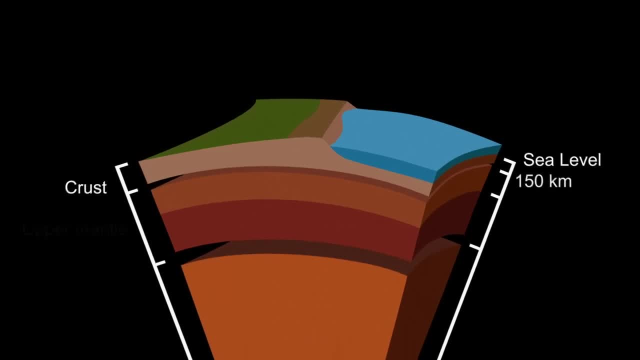 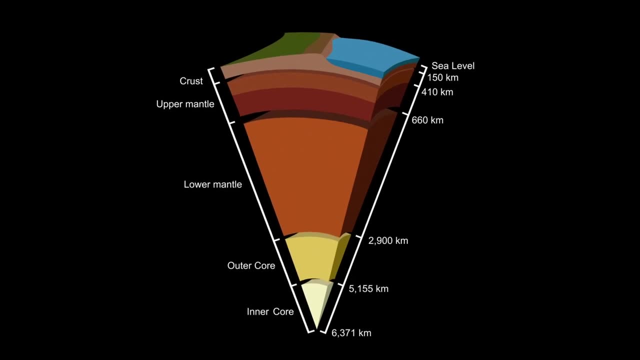 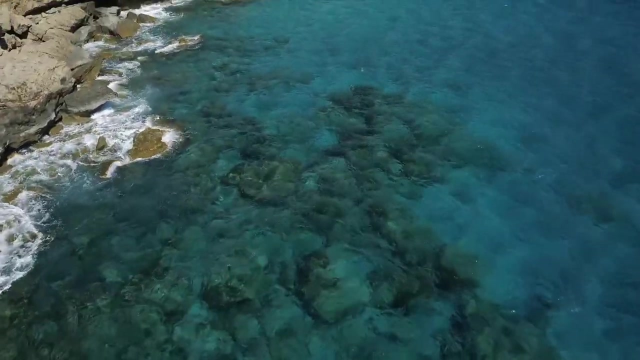 While the crust may seem incomprehensibly thick, in reality the Earth's crust is very thin when compared to the rest of the Earth's layers. The Earth has two types of crust: Oceanic crust, which makes up the ocean floor, and continental crust. 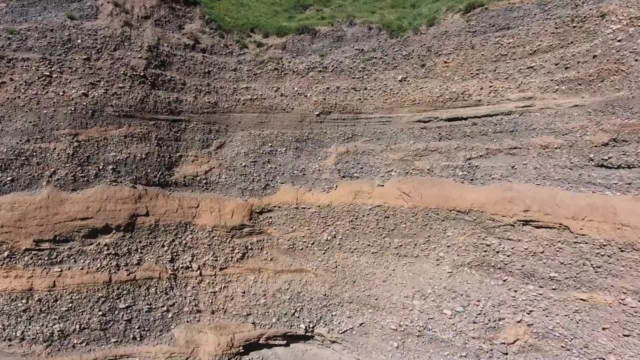 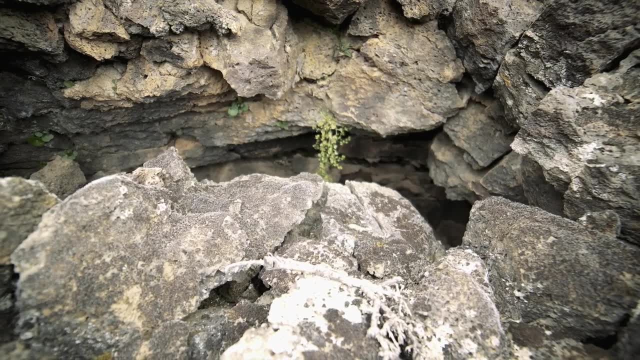 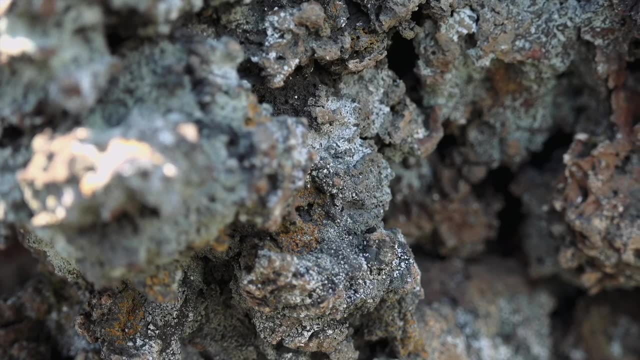 which is the crust that forms land. Each type of crust is made up of many different types of rocks and minerals. In the oceanic crust, In the oceanic crust, In the continental crust, which is about 6 to 7 kilometers or 3 to 4 miles deep, we find basalt rock formed by the rapid cooling of lava. 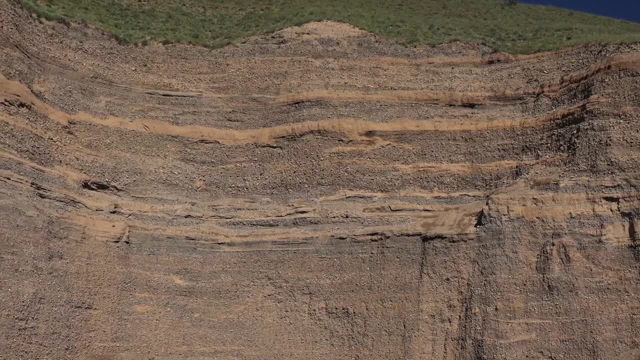 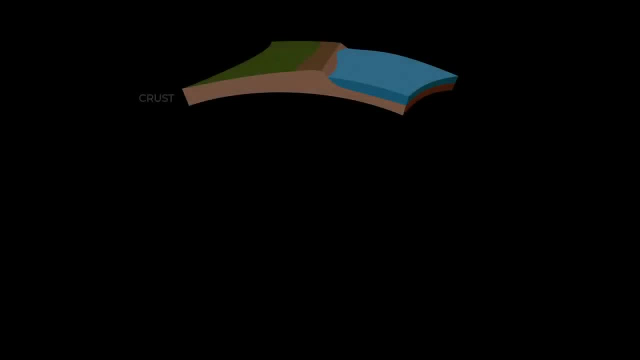 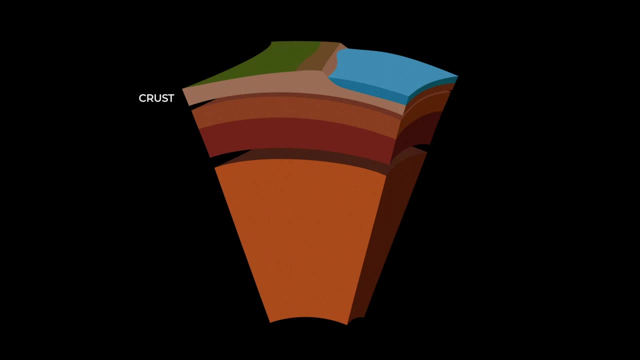 In the continental crust, which is about 38 kilometers or 25 miles deep, we find granite, the most common rock in the Earth's crust. Just below the crust is the mantle, which is also made of rocks and minerals. The mantle is separated into two layers: the upper mantle and the lower mantle. 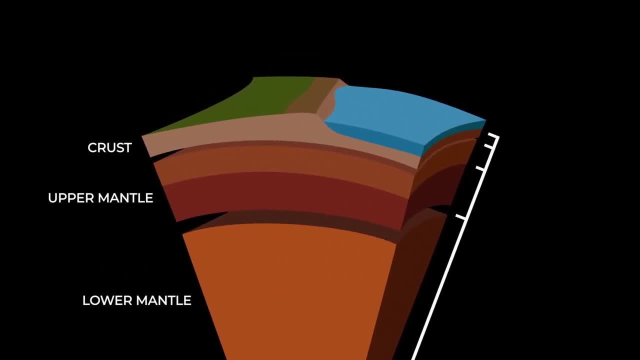 The upper mantle, which is closer to the Earth's crust, has lower pressure and cooler temperatures than the lower mantle. Though it is cooler, the upper mantle still ranges from 1,400 to 3,000 degrees Celsius, or 2,500 to 5,400 degrees Fahrenheit. 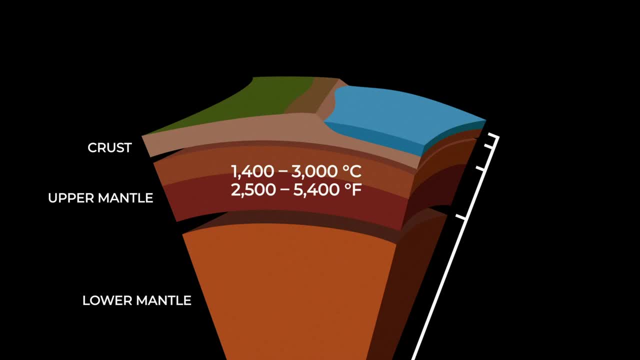 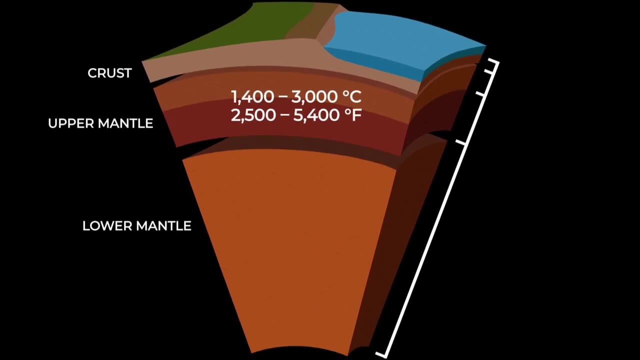 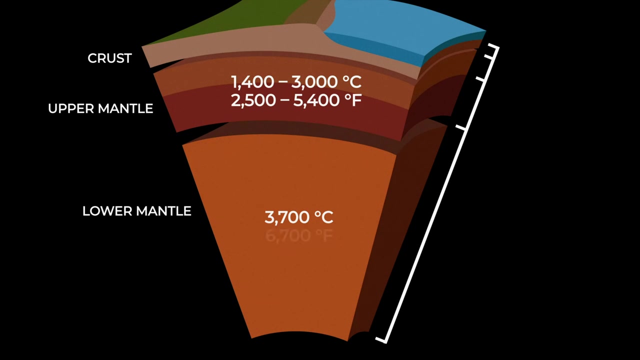 As a whole, the mantle is in a solid state. However, the topmost part of the upper mantle is composed of hard rock, whereas the bottom part of the upper mantle has both hard rock and soft rock that bends and flows. The lower mantle, which rests beneath the upper mantle, reaches temperatures of 3,700 degrees Celsius or 6,700 degrees Fahrenheit. 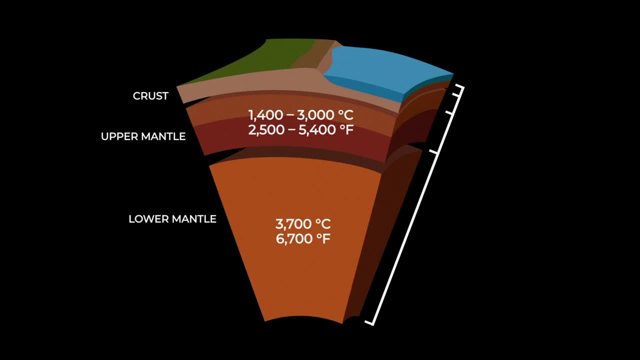 Though it's hot enough to melt rock, it doesn't. It stays solid because the pressure is too high. The pressure of the rock is too high to allow the rock to melt. Overall, the whole mantle reaches a depth of 2,900 kilometers, or about 1,800 miles. 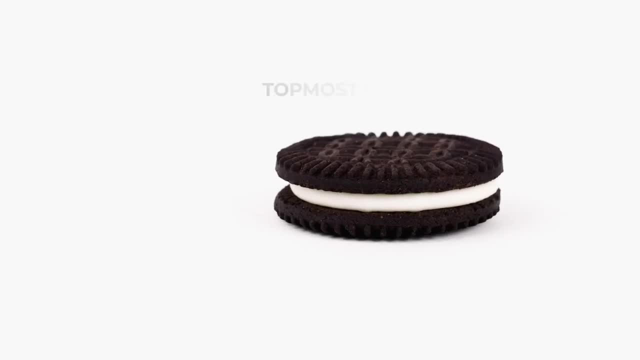 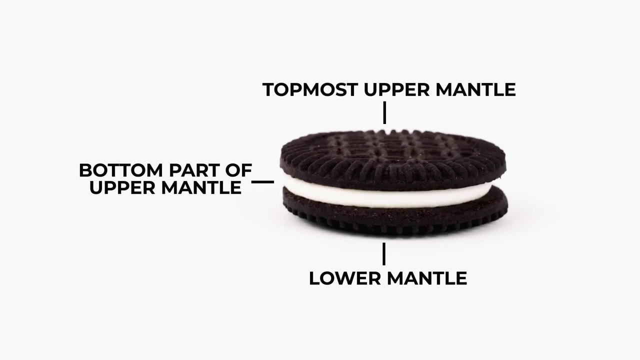 You could think of the mantle as a sandwich cookie, where the top hard cookie is the topmost part of the upper mantle. The soft cream layer represents the soft bendy rock found in the bottom part of the upper mantle. Finally, the bottom hard cookie is the lower mantle. 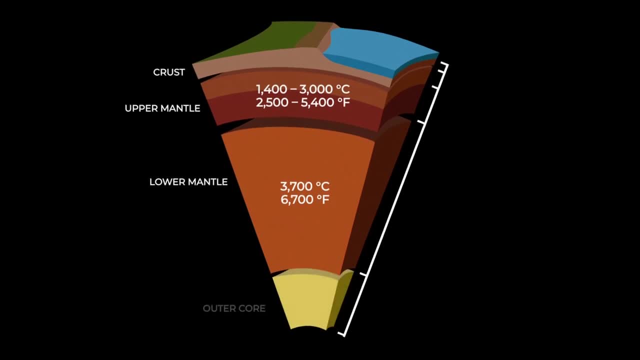 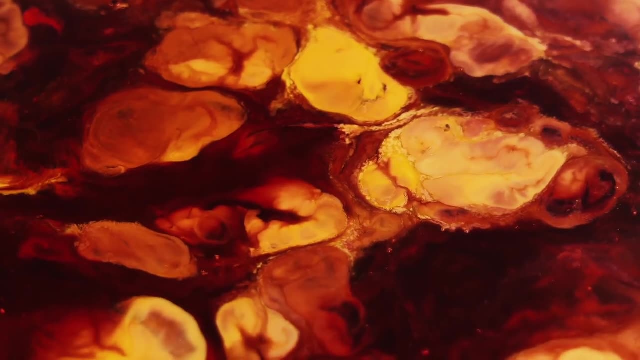 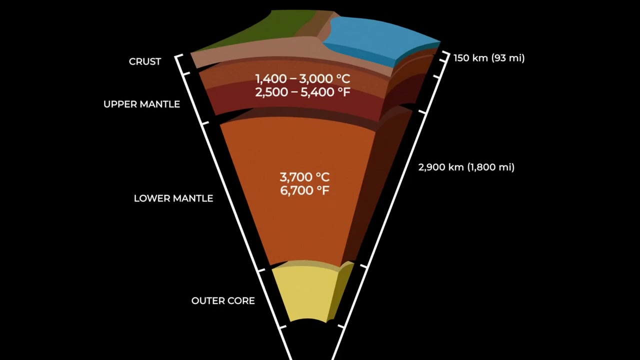 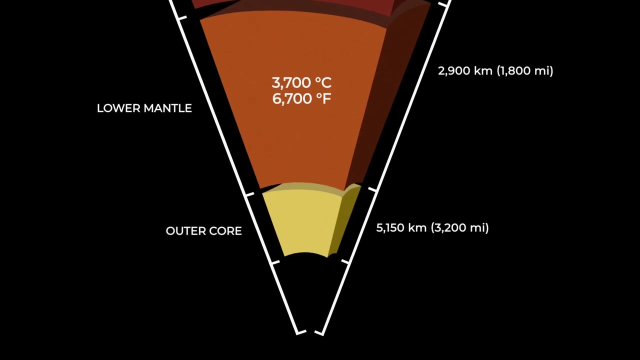 Travelling past the mantle, we reach the outer core of the Earth. This layer is liquid and, because it is made mostly of a combination of the metals iron and nickel, it generates a magnetic field that surrounds the Earth. The outer core, from the bottom of the mantle, extends to a depth of 5,150 km or 3,200 miles.